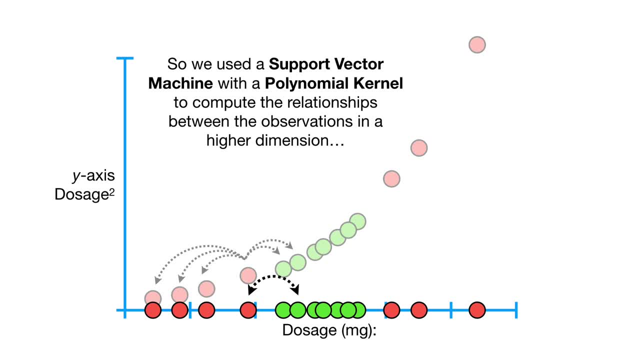 So we used a Support Vector Machine with a Polynomial Kernel to compute the relationships between the observations in a higher dimension and then found a good Support Vector machine that could be used to compute the relationships between the observations in a higher dimension, and then found a good Support Vector machine that could be used to compute the relationships. 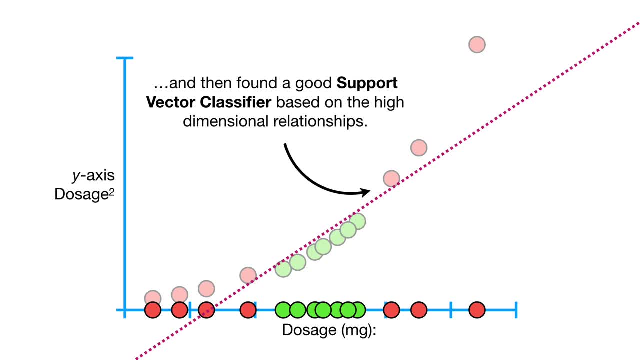 between the observations in a higher dimension and then found a good Support vector classifier based on the high-dimensional relationships. The Polynomial Kernel that I used looks like this: a and b refer to two different observations in the dataset. r determines the coefficient of the polynomial. 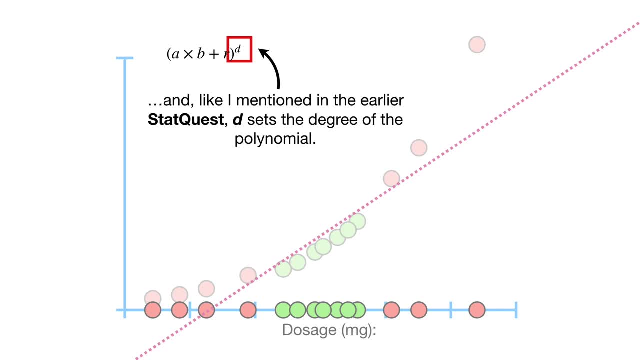 And, like I mentioned in the earlier StatQuest, d sets the degree of the polynomial. ii sets the degree of the polynomial. It depends how much you set for that. In my example I set r equals one for Bush v and it says how much. what's drag equal to. 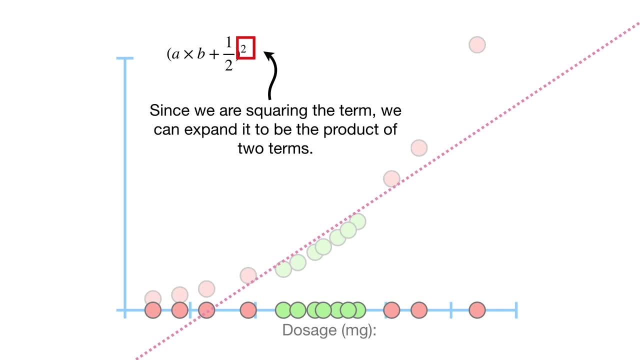 1, half and D equals 2.. Since we are squaring the term, we can expand it to be the product of two terms. Now we just do the multiplication and combine these two terms. And just because it will make things look better later, let's flip. 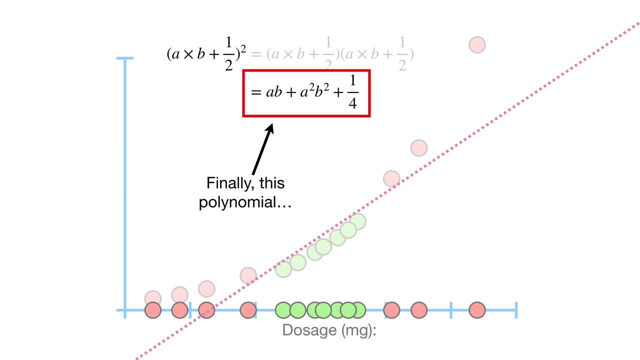 the order of these two terms. Finally, this polynomial is equal to this dot product. A dot product sounds fancy, but all it is is the first terms multiplied together plus the second terms multiplied together, plus the third terms multiplied together. The dot product gives us the high dimensional. 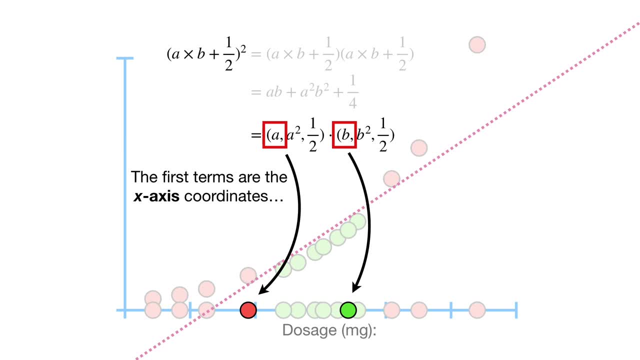 coordinates for the data. The first terms are the x-axis coordinates and the second terms are the y-axis coordinates. The third terms are z-axis coordinates, But since they are the same for both points, we can ignore them. Thus we have x and y-axis coordinates for the data in the higher dimension. 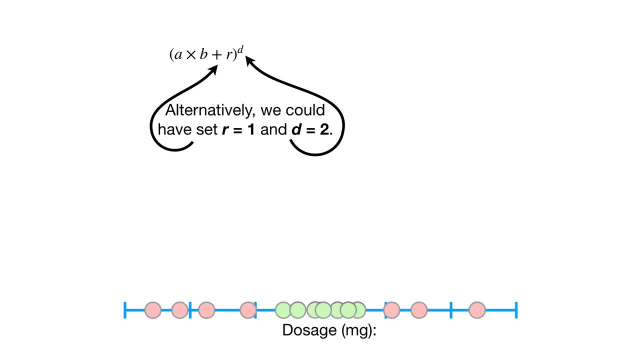 BAM. Alternatively, we could have set r equals 1 and x equals 1. And D equals 2.. Now when we do the math, we get this polynomial and this dot product. We can verify that the dot product is correct by multiplying each term together and then. 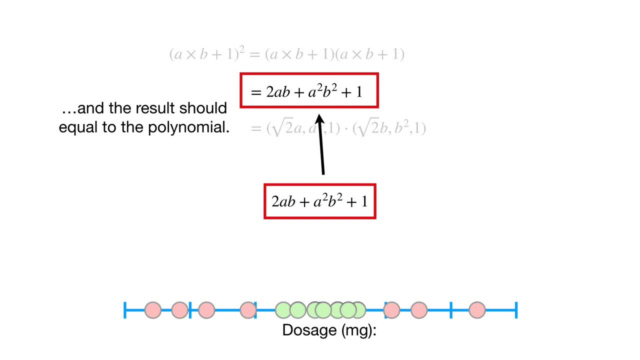 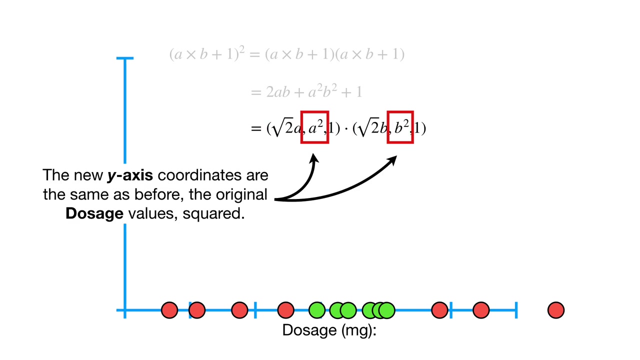 add everything up and the result should be equal to the polynomial. Using this dot product, the new x-axis coordinates are the squares. The new z-axis coordinates are the square root of 2 times the original dosage values. So we move the points on the x-axis over by a factor of the square root of 2.. 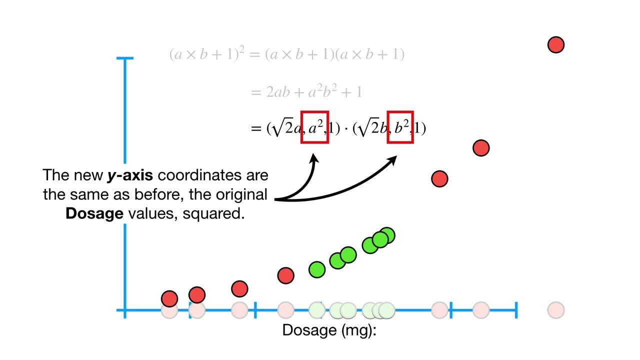 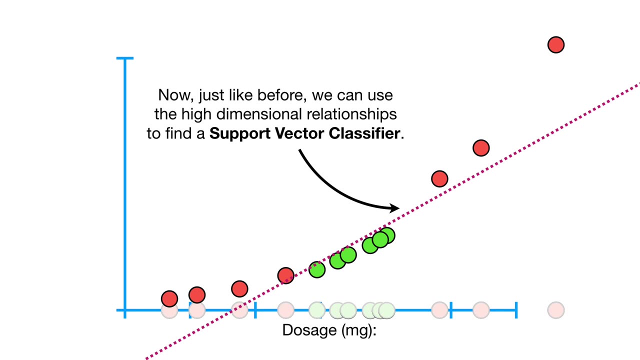 The new y-axis coordinates are the same as before, the original dosage values squared And, just like before, we can ignore the z-axis coordinate, since it is a constant value. Therefore, we can use the high-dimensional relationships to find a support vector classifier. 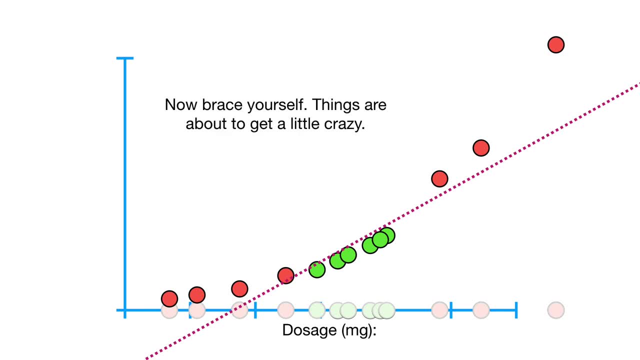 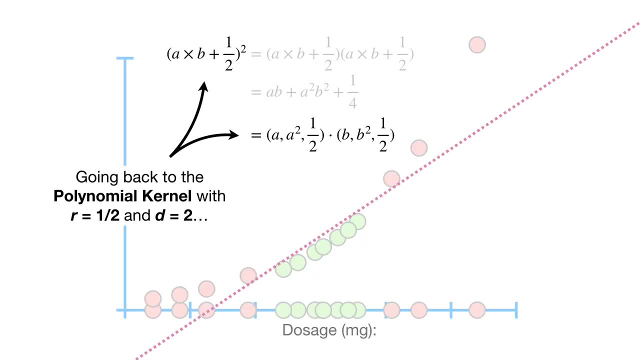 Double bam. Now brace yourself. things are about to get a little crazy. Going back to the polynomial kernel, with r equals one-half and d equals two, it turns out that all we need to do to calculate the high-dimensional relationships is calculate the dot products between each pair of points. 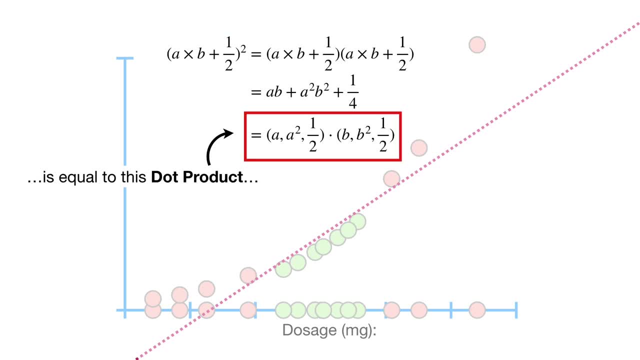 And since this kernel is equal to this dot product, all we need to do is plug values into the kernel to get the high-dimensional relationships. For example, if we wanted to know the high-dimensional relationships between these two observations, then we plug the dosages into the kernel, do the math. 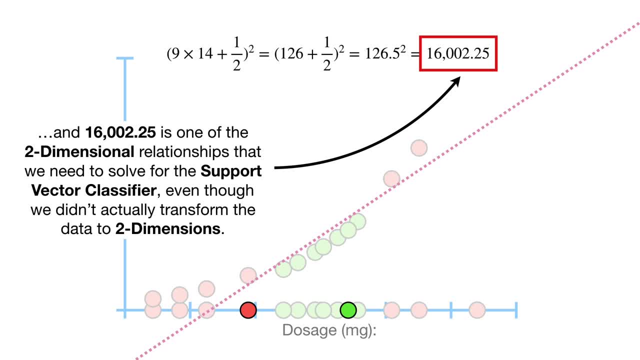 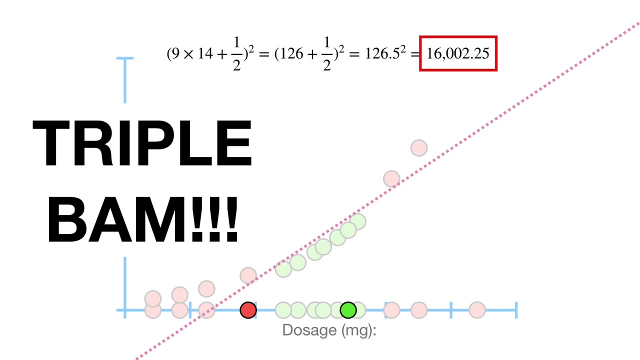 and say that r equals one-half and d equals two. 16,002.25 is one of the two-dimensional relationships that we need to solve for the support vector classifier, even though we didn't actually transform the data to two dimensions. Triple bam. 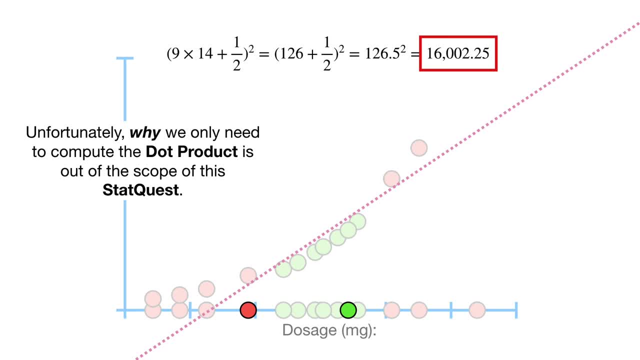 Unfortunately, why we only need to compute the dot product is out of the scope of this stat quest. Wah wah. To review the polynomial kernel is a very simple function. The polynomial kernel computes relationships between pairs of observations. A and B refer to the two observations that we want to calculate. the high-dimensional